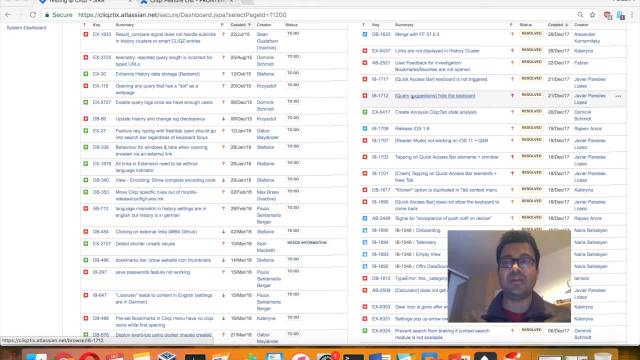 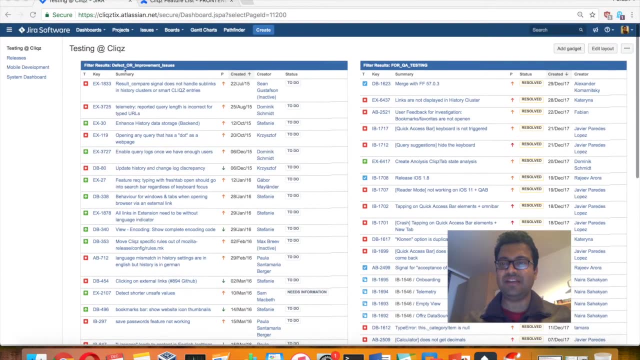 So in today's presentation we are going to learn all these three things together. So here we go. You can see my screen and I am logging to Jira software. So you have two kind of versions for Jira available in the market. Either you can use the free version- it has certain limitations- and other one is the licensed one. You can pay and get a license for you and your team. 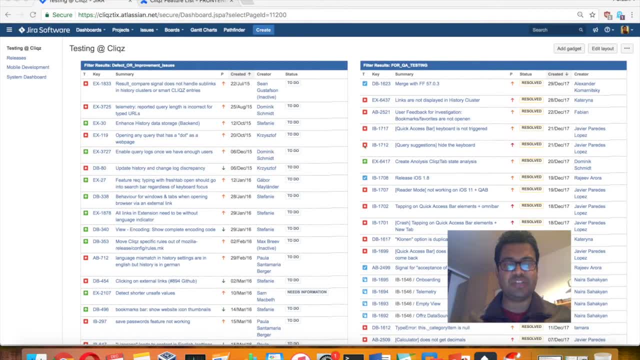 So this is the free version. This is what you are seeing over. here is a dashboard which has been created by me. We will cover dashboard in my upcoming sessions on Jira. Today we will talk about defect life cycle management. So, friends, as you know, defect is something. it's a kind of issue or bug, or whenever you see any deviation from expected behavior, or if you have a business requirement. 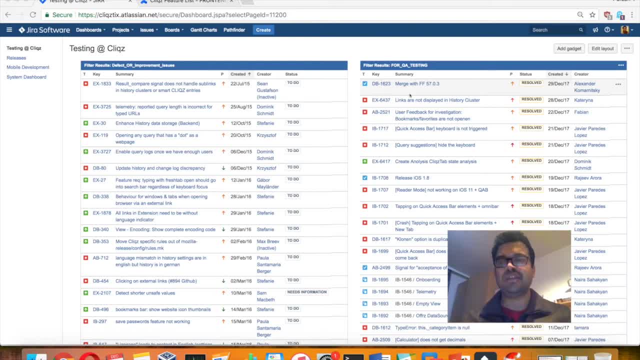 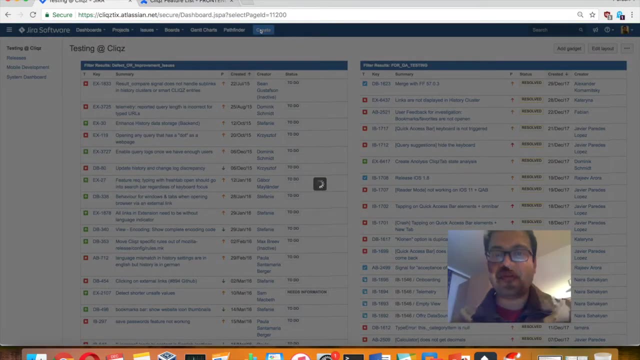 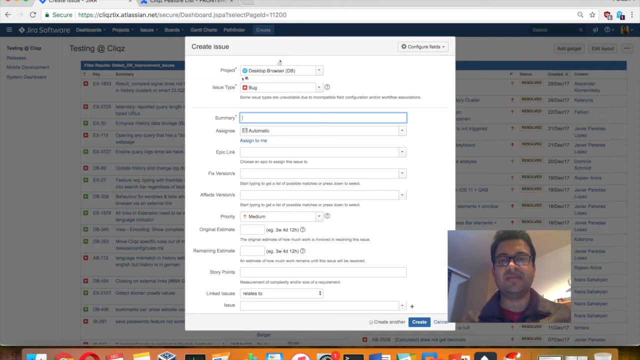 or if the actual behavior of the software or service is not matching to the expected one, then we see this deviation is a defect. So first of all, when a defect is observed, it has to be reported. And how we do it? We do it as a part of defect creation process. You can see I clicked on this create button. As soon as you click on create you get to know about you have to fill in certain fields. 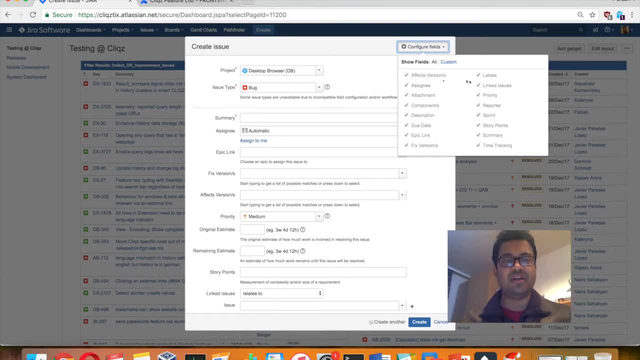 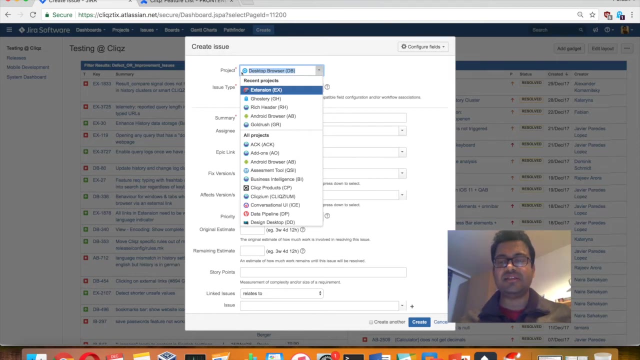 These fields can be configured from here. So these are the fields which are to be entered whenever a user is inputting or providing details about the defect. So let's see, I have to put in the kind of project, which project this defects belongs to. 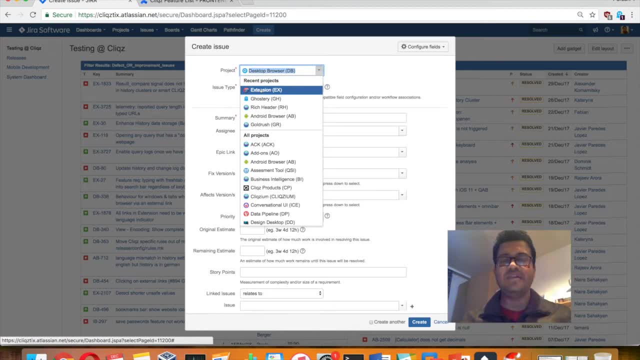 So, if you have a defect, what would be the project in which I can put it and where this defect is impacting? What is the impacted area? Depending on that we put in the project. You have issue types. Issue can be anything. It can be an improvement, You see, a business improvement or functionality improvement. It can be a dev task, QA task. 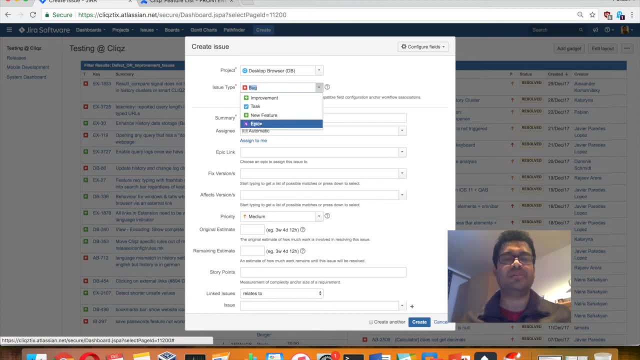 You see, it's a new feature or it might be an epic on which everybody is going to work. So the kind of feature which I'm feature or the fields which I'm explaining over here, they are from agile project And more or less these are interchangeable. So maybe traditional or agile or any other mode of project management. 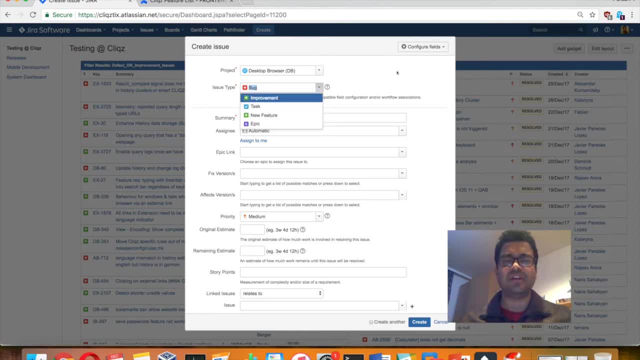 You can. you can freely interchange the kind of field and you can configure them. You can ask your Jira admin. There's always a Jira admin who can go ahead and give you access, depending on which you can either write or edit, or even just view. 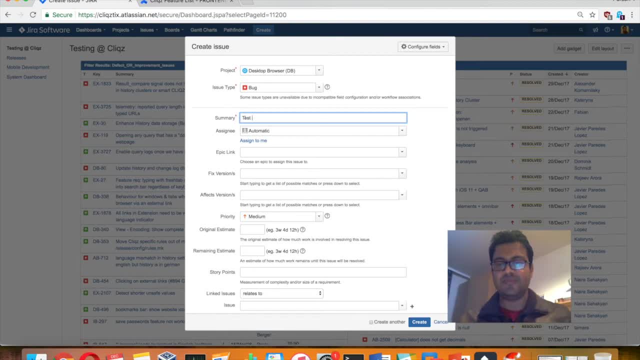 Here you provide in the summary. This is just a normal one. You can give in a detailed summary, like I can see: console exception seen when launching the service or launching the product and the system is crashing. You can give something like this, which is summary. You can provide the name of a signee. 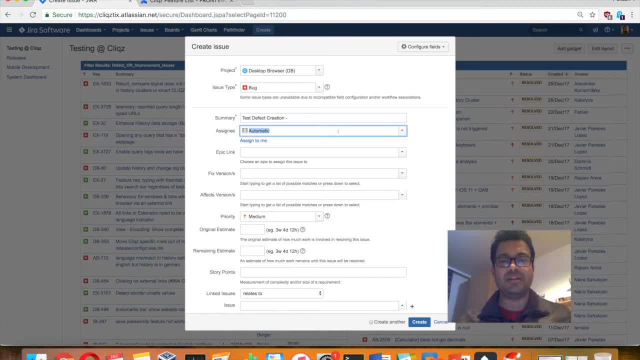 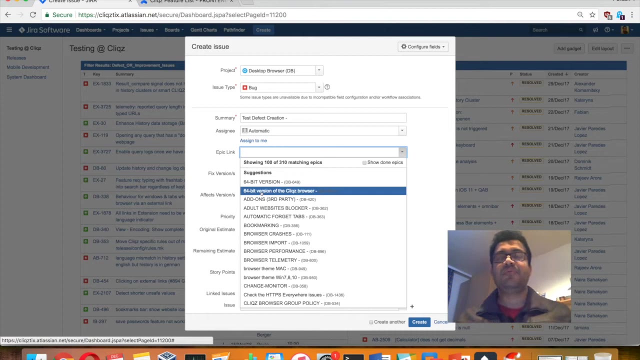 Everybody who is in the project. they'll be automatically populated in this signee letter, For example, if I see my name. So all those people who start with this, you can provide their name in the signee factor. Epic is something. if it belongs to any of the epic- a very big requirement which was in development- then you can provide the epic. 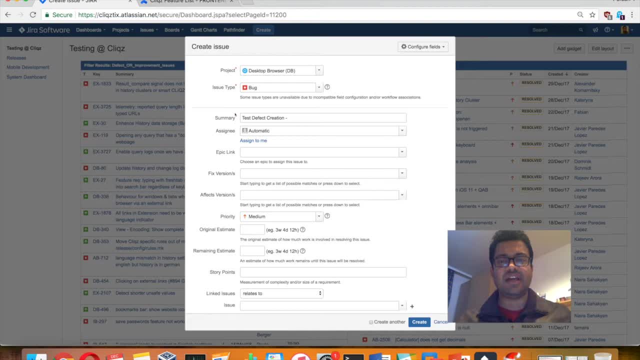 It is non-mandatory field. Anything which is with a star is a mandatory field. So you have to fill in those star rated fields because it is a very important information Which the signee or the reporter may or may not remember at the time of fixing or reproducing the issue. 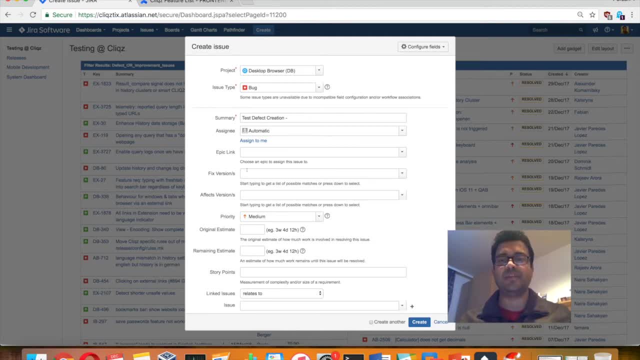 So these fields with the stars are the most important ones. You have fixed version. What is the version in which you want this defect issue to be fixed? And then you give the affected version. What would be your affected version, For example? I can select you have. these are the different released and unreleased version. 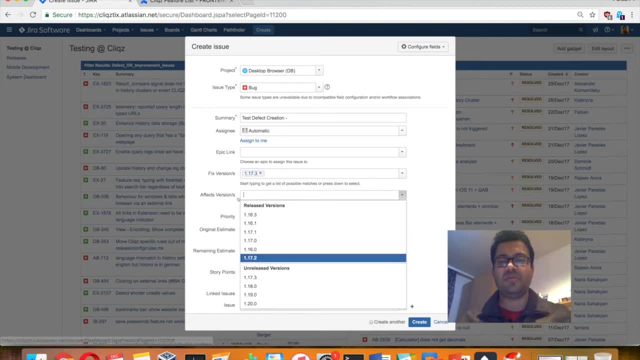 I can select any one of these And I want it to be. it is affected version, whether affecting the previous version, and I want to get it fixed in the upcoming version 1.17.3.. What would be the priority? So most of you, whenever you raise a defect, you know we have a priority of defect. It can be high, medium or low or critical, But depending upon how much your defect is impacting the system, Depending on that you can give this high, medium, low, critical- whatever criticality or priority Original estimate. you don't have to fill it. 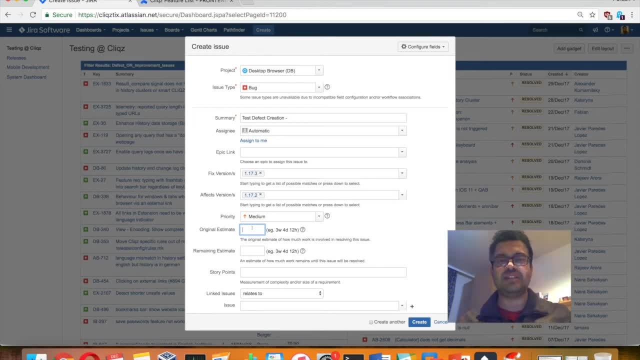 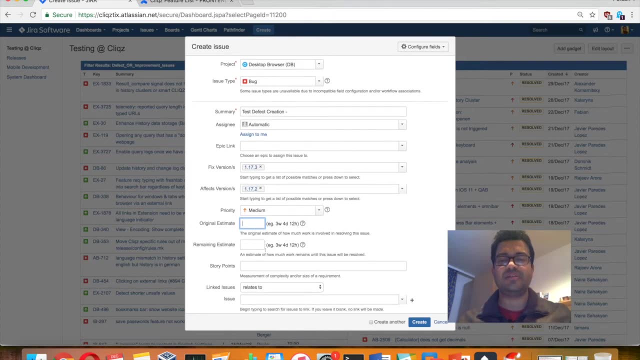 This can be used by developers whenever they see, or support team whenever they see this issue. They can set their own deadline and provide estimate, And this will give a remaining estimate. whatever it is Story point is used for estimation. You don't have to worry about it. 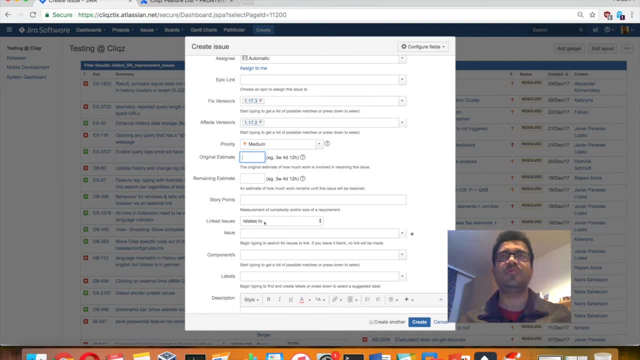 Linked issue. if, in case, this issue was there and you want to relate it with something which was observed in past, Then you can relate it over here. Or you can say: this is a clone, This is cloned by some other issue which was there in past. 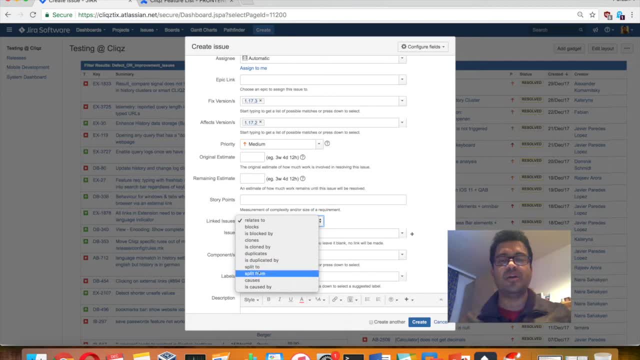 It is a duplicate, Or you can split into two parts, Or it is coming from some other issue. It is caused by some other issue. So all those things you can provide it there. You can give the Jira ID of the other issue. 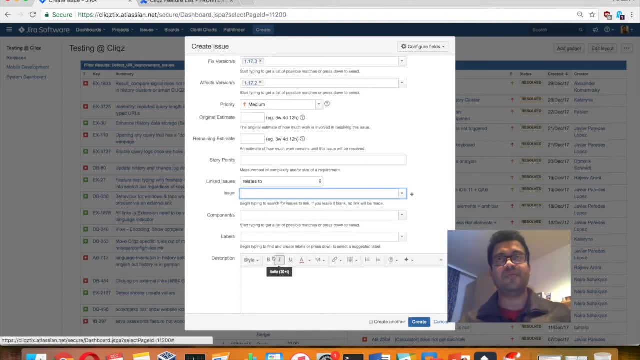 Components, you don't have to worry. Component is something. if you are an automation tester or you know the system very well And you know which component may be business component, may be technical component which is getting impacted, You can put it over here. 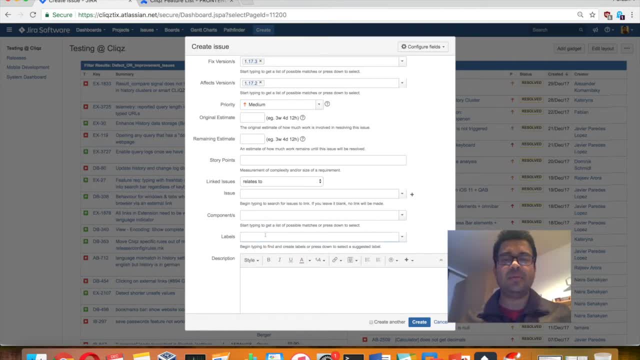 You can create a separate label, Like at any point of time you want to segregate all those issues which are having a label. It is very easy: You just go and click on that label and all those Jira issues which are there with this label, they will be listed together. 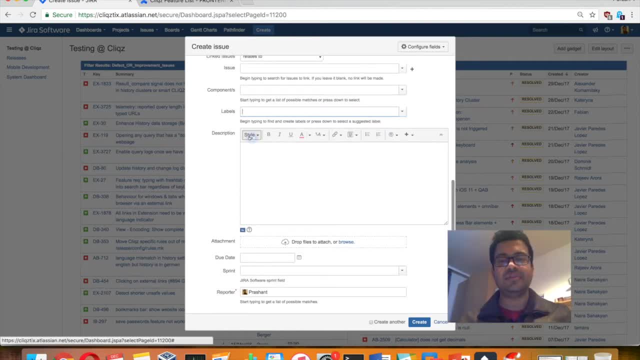 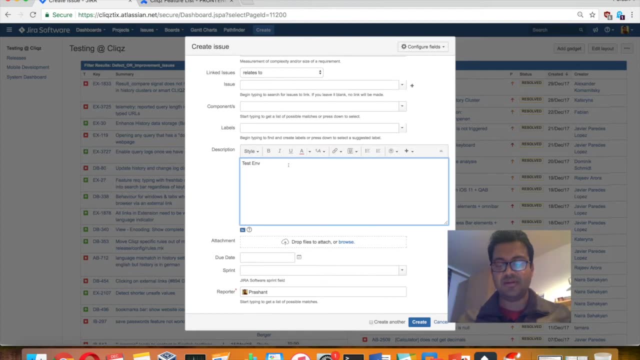 And here you need to provide in a description. Description should be detailed, Detailed, like, for example, your test environment, Your testing steps to reproduce And then you can provide in anything like in exemptions Plus you have any kind of specific requirement, like it was tested in system testing or integration testing or regression testing. 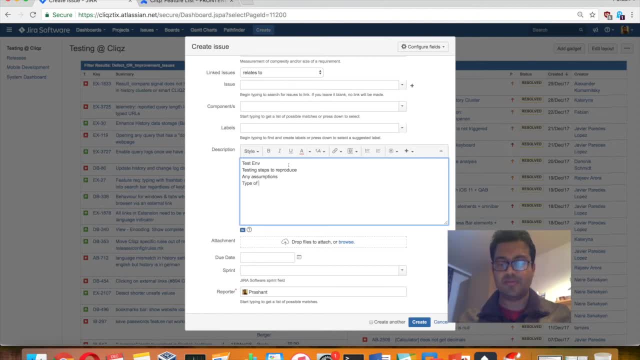 So anything like that can be flashed. This thing is great. Plus, if you want, you can put in the version of where it was working. It is the expected result And then you can actually insert. Plus, you need to provide any screenshot or logs. 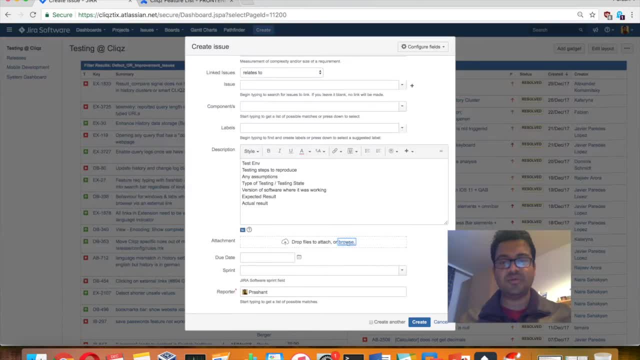 You can go ahead and provide any kind of screenshots or logs. Just go ahead and attach it to this Due date. you don't have to worry Project managers: if they want, they can put in a due date And, depending on the due date, they can follow up and see where the issue is. 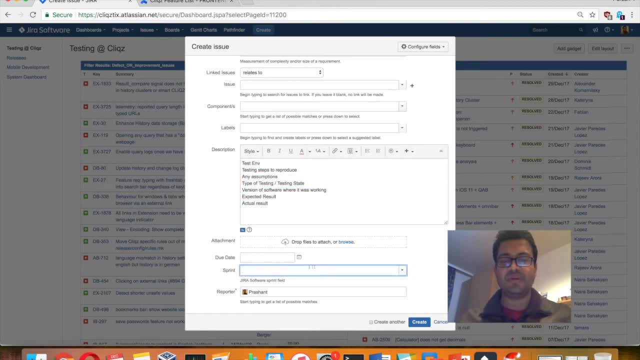 If you want to put it into any kind of a sprint, go ahead and provide the sprint And here the person who is creating his name will be over here As the port type you want. you can change it to somebody else's name. 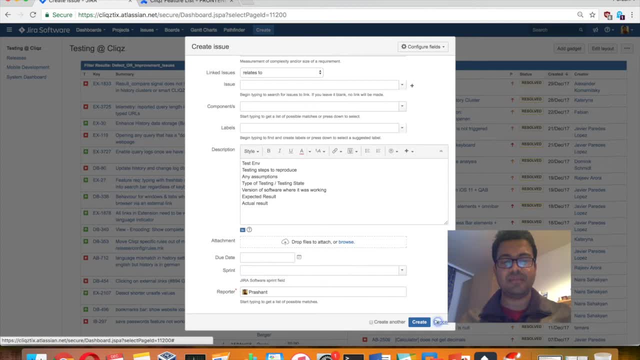 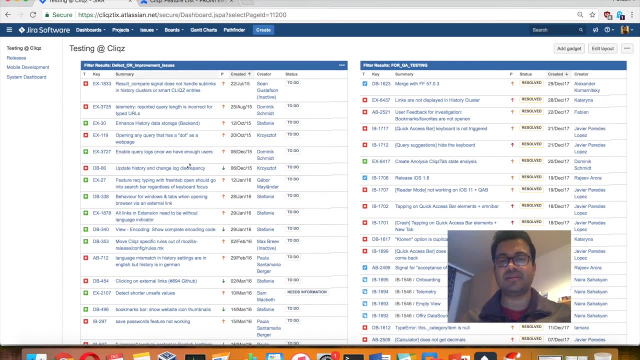 And as soon as you click on create, defect is created, Canceling it now, And, let's say, a defect is created, something like this: So this is my board, I'll open. I'll go ahead and open one of the issues. 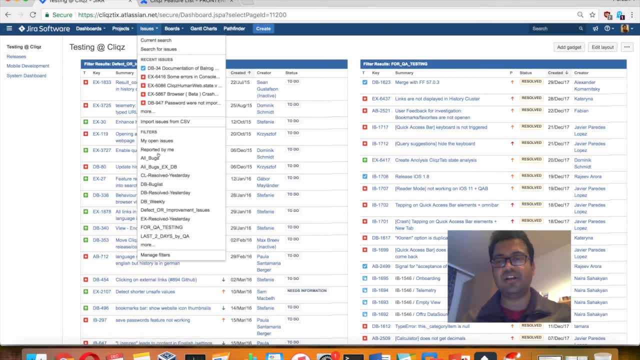 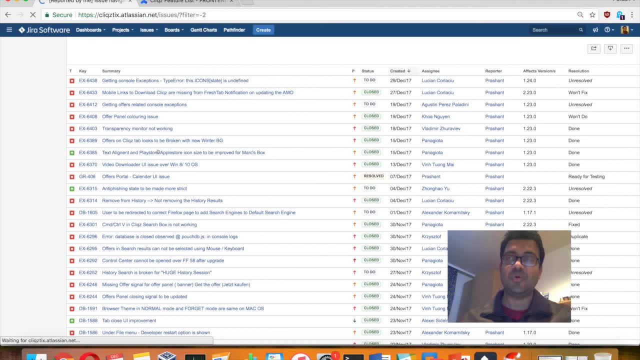 My reported by me. These are the different kind of filters which I have been using, reported by me. Some are default and some you can create on your own. If you are interested to know how to create filters, please let me know. I'll come up with a next video. 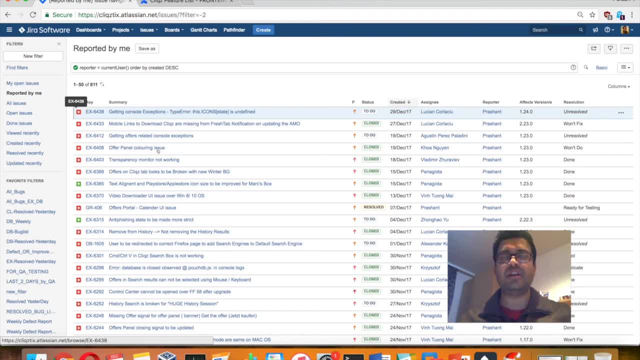 I don't want to make this video pretty long enough, So I'll come up with the next video wherein I'll provide any kind of answers, what you people are looking for, If you want to know anything about Jira in an enhanced manner, or any specific thing which you want to know, like 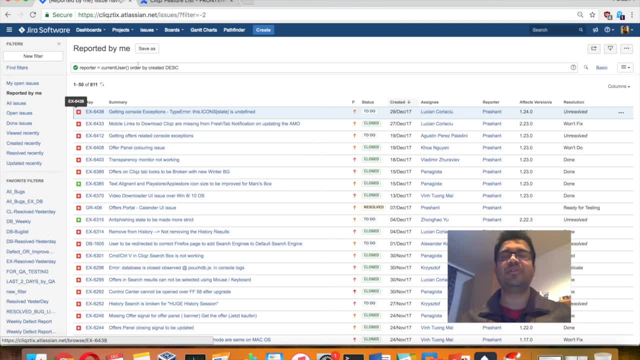 let's say, creating dashboards or using the widgets or managing different kind of users. Please let me know in your comments for my video, and I'll surely go ahead and make a video on that thing as well. So let's say, these are the issues which have been raised by me. 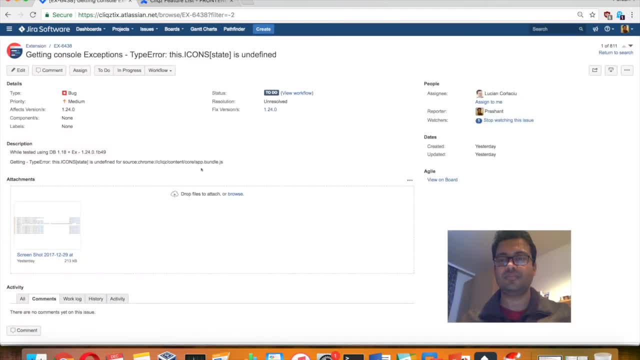 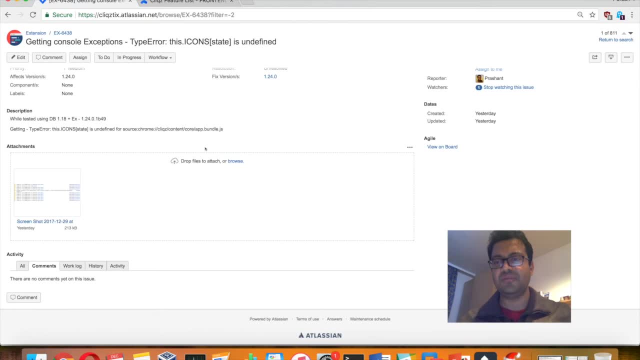 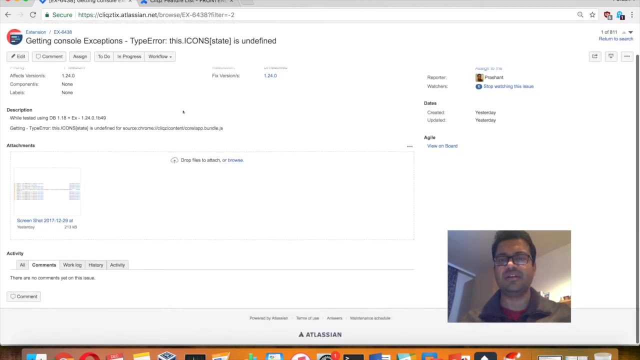 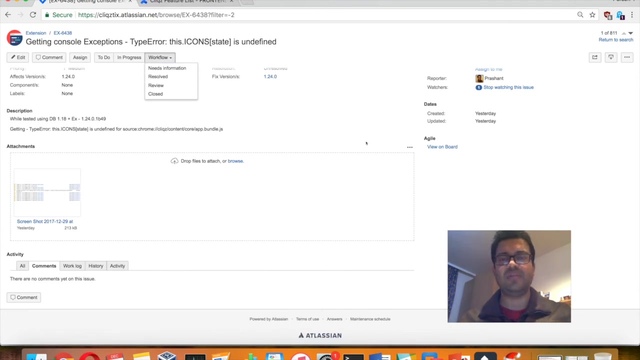 So this is just a normal issue which has version and some information which I have raised, And it was about the console exceptions, what I was getting. So you see, there is a workflow And I can, once it is done, developer, it is assigned to a developer that this developer can mark it as resolved. 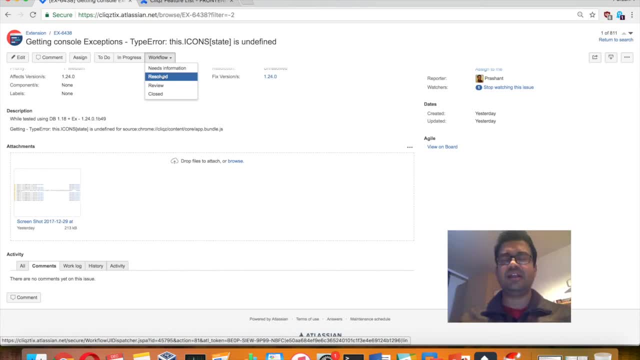 So whenever you raise a defect, that defect the next stage is it is assigned to a developer Developer. then try to reproduce it. If he sees it is a valid defect, he can go ahead and fix it. If developer thinks the defect is irrelevant or something which is not important, he will put his comment, mark it as resolved or close it. 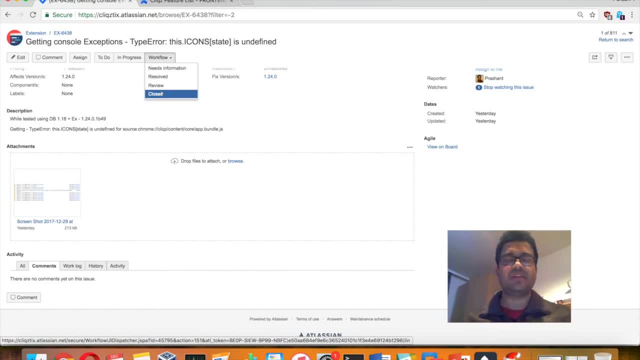 And then it is just taken out of the system. It can be marked as closed. But if he is working on it, then at any point of time you can mark it as need information And then it may be requiring any kind of information from the reporter or somebody else who is like designer or somebody else who is involved in the development process. 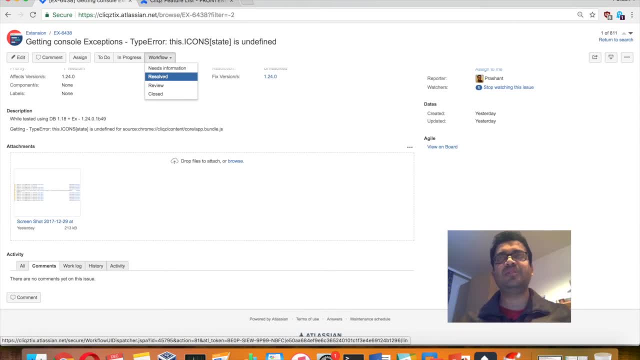 And then, once it is done, the mark it as resolved. Once it is resolved, it is moved back to the tester And tester they go ahead and pick it up again, make it as ready for testing. Once it is ready for testing, they go ahead and mark it as either closed or not closed. 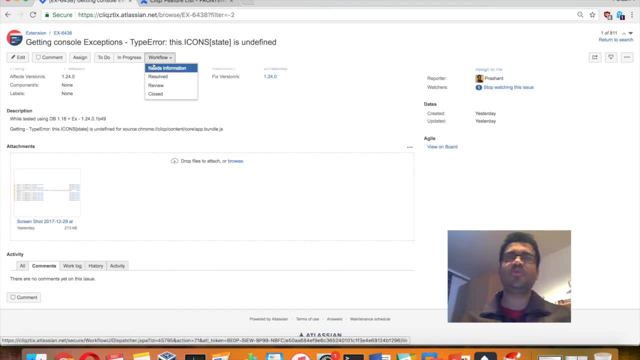 If they say it is not closed, they will mark it as to do. And then to do is the state which is like ready to be developed or ready for development, And as soon as a developer starts working on it, they mark it as in progress. And once it is done with the development, once they are done with the development of fixing the bug, they mark it as resolved. And once it is resolved it is taken by testers and it is ready for testing Tester. depending upon the bandwidth or the kind of testing they are doing, they can pick it up and check it on the latest version. 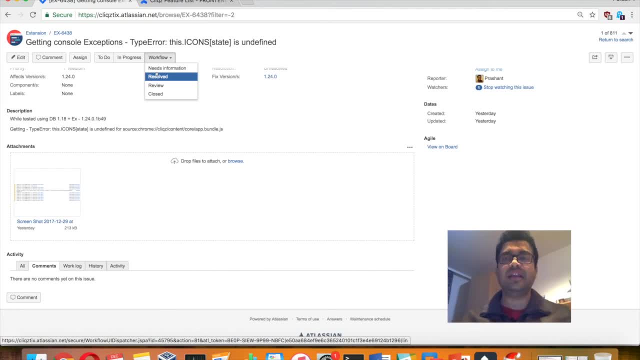 If it is fixed, they will say: while testing, they will mark it as in test And once it is tested they can mark it as closed or reopen and assign it to developer. So this is the way we create a complete defect lifecycle flow in Jira.